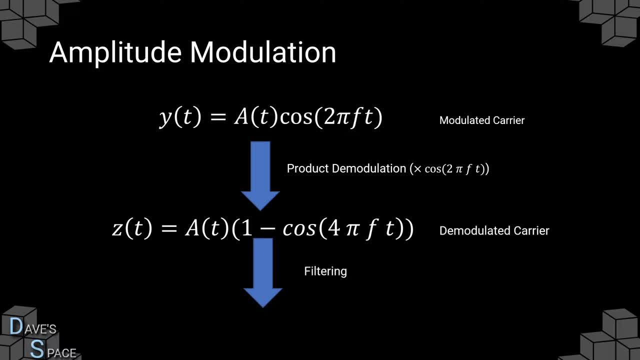 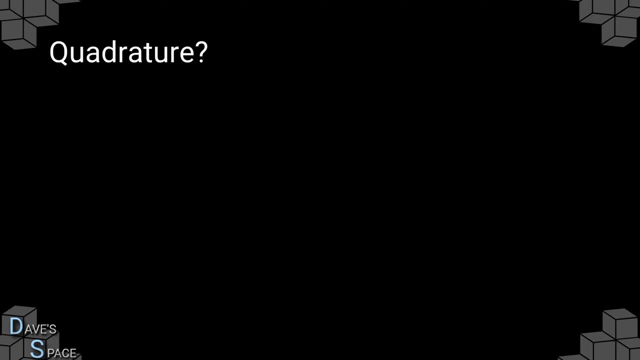 demodulated carrier. we can then apply some filtering to the high frequency components. we should then leave us with a signal that's roughly equal to the original modulation waveform aft. and so how do we add quadrature components to our amplitude modulation? but what does quadrature mean? quadrature, very simply. 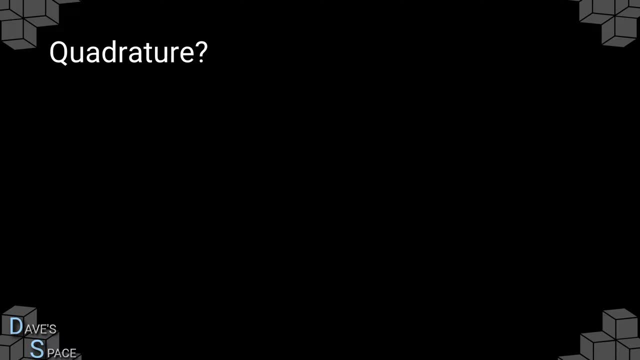 means two signals which are out of phase, by plus or minus 90 degrees or plus or minus pi over 2. so for example, sine and sine of X, plus or minus pi over 2, are two quadrature waves. likewise cosine and cosine plus or minus pi by 2 is also a. 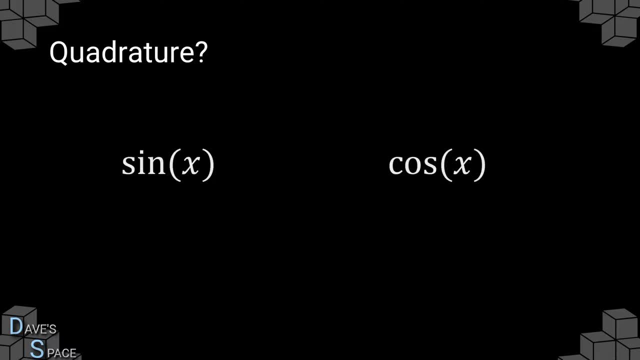 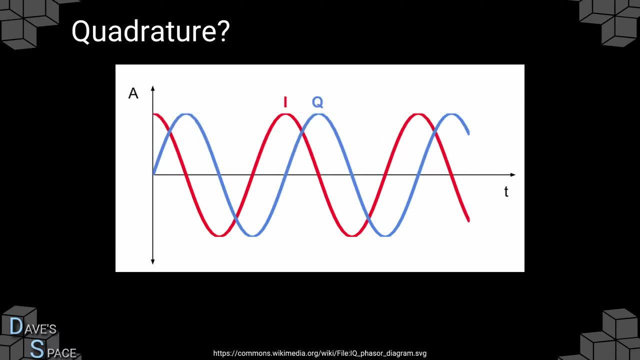 quadrature signal, and so naturally, sine and cosine are two signals that are in quadrature, and this can be shown on a graph like this. you can see how the waves are the same: they are 90 degrees out of phase with each other. and so what happens if? 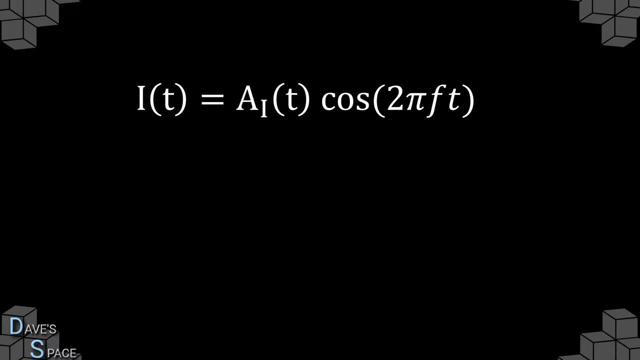 we take an amplitude modulated signal, which here we'll call I of T, which consists of a modulation waveform, AI of T, multiplied by the cosine of 2 pi f of T, where F is our carrier frequency. what happens if I take another modulated waveform, here Q of T, with a different? 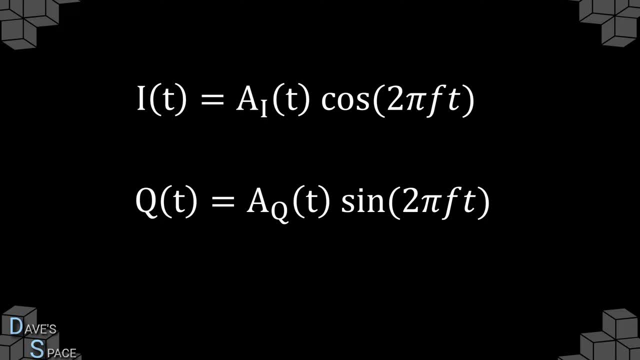 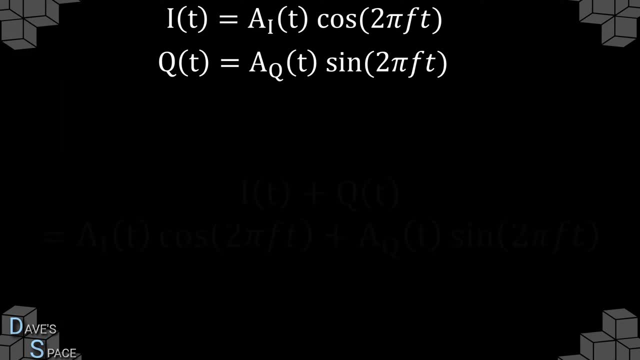 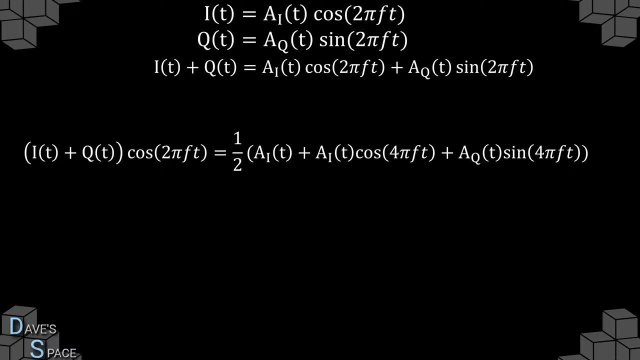 modulation waveform: a of Q, but now multiplied by sine of 2, pi, F of T. if we then add those two signals together, we get something very simple which is just the addition of the two. now the trick with these quadrature signals is to realize that if we multiply the summation of the two quadrature signals, 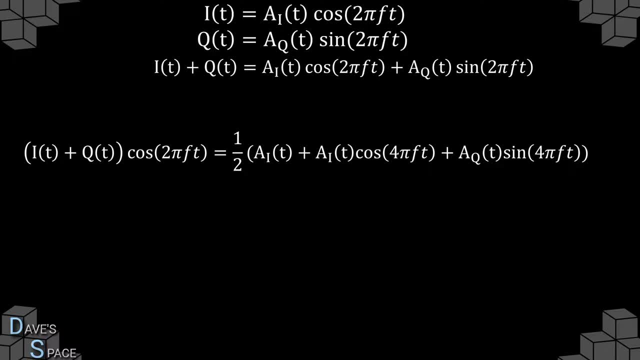 by cosine 2, pi F of T. what we end up with is the expression. here you'll notice that we have a constant expression, AI of T, which was the original modulation waveform of the cosine component I of T, multiplied by some high frequency oscillations at twice the original carrier frequency. likewise, if we 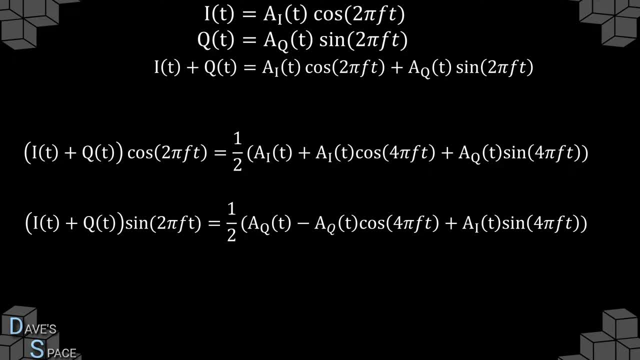 multiply the same I plus Q of T by sine of 2 pi F of T, what we end up with is a constant AQ of T, which was our original modulation waveform for the sine component Q of T, with some more high frequency oscillations. and so it stands. 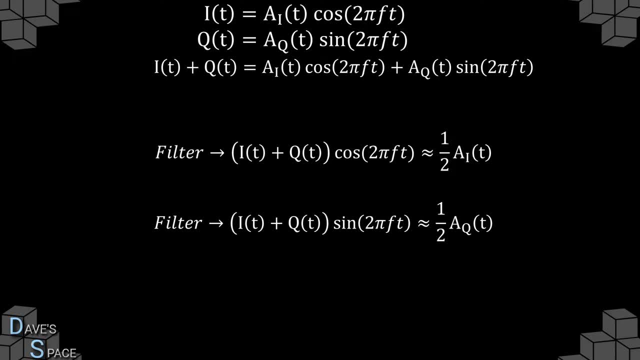 to reason that filtering those signals should now lead us to be able to recover our original modulation waveforms A of I and A of Q. so, even though we start off with two separate signals, cosine and sine, multiplied them independently with some modulation waveforms, upon doing coherence, demodulation, in which we 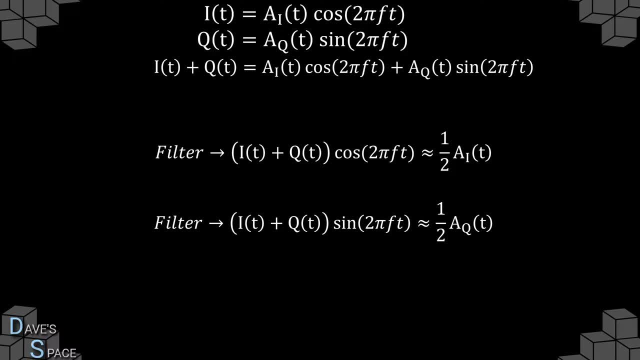 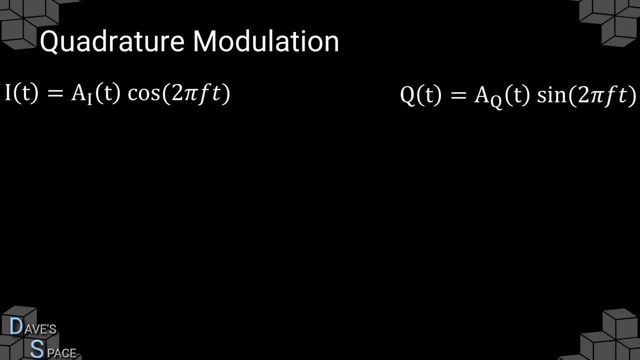 multiply 1 by cosine and 1 by sine, we can recover our original signals, and so the process for quadrature amplitude modulation goes something like this: we start off with our two modulated carrier waves and then we add them together. we can then send this out. once our signal is sent out and received, we can take. 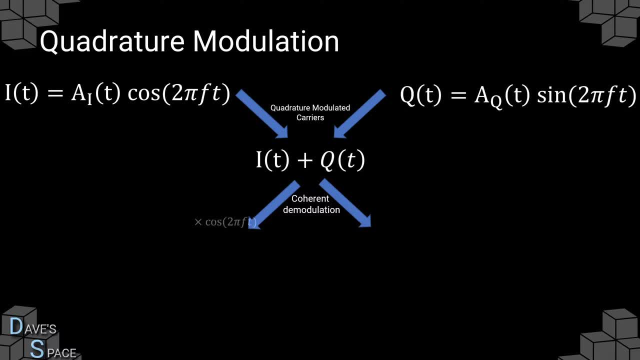 that signal and coherently demodulate it, in which we can multiply it by cosine of 2 pi F of T and sine of 2 pi F of T. in each case, we recover the amplitude modulation signal applied to each of the original carrier waves. what's important? 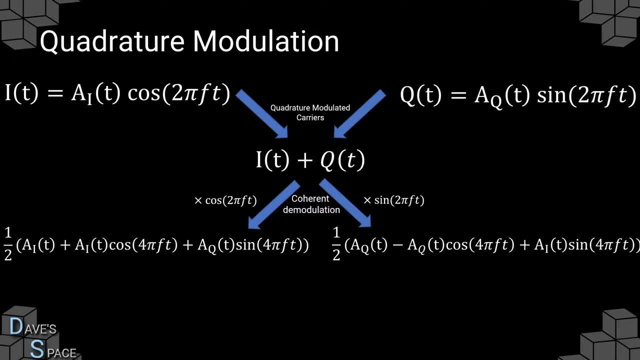 to note here is that the demodulation is coherent, so we must multiply by cosine and sine for the original carrier wave. now this is very important is that then we need to know the exact phase of the original wave, otherwise we will not be able to extract our original AI and AQT signals. 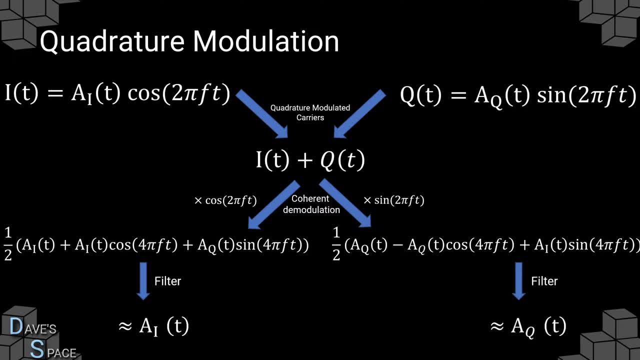 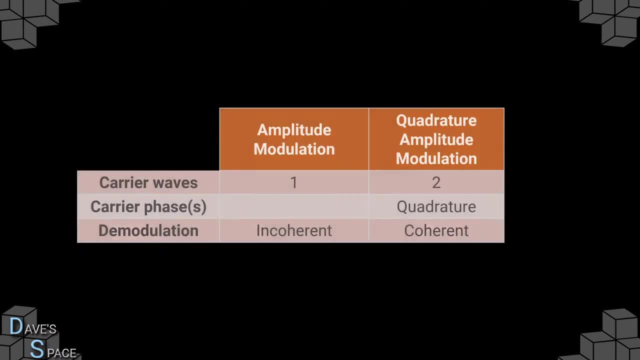 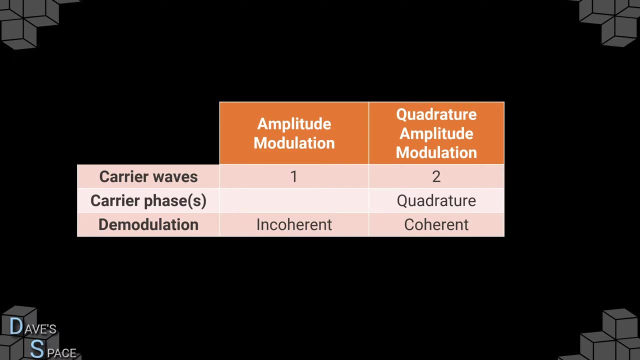 the last step is to filter the signals which to give us a good approximation to the original modulation waveforms. and so just to look at the differences between amplitude modulation and quadrature amplitude modulation: for amplitude modulation we only have one carry wave and for quadrature amplitude modulation we have two. the carrier phases must be: 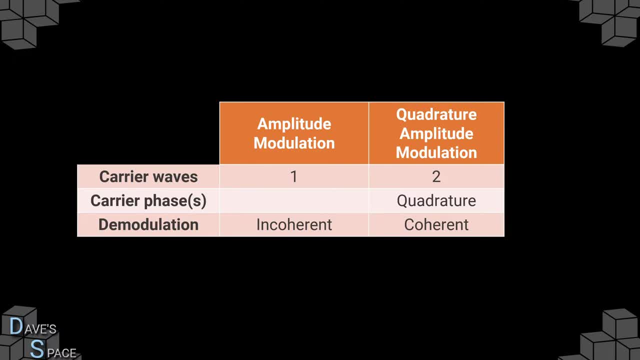 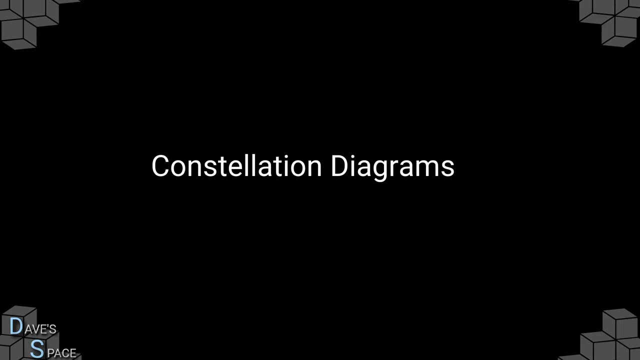 in quadrature. for the quadrature amplitude modulation and the demodulation must be coherent. for the quadrature amplitude modulation there is no such restriction on not regular amplitude modulation for coherent demodulation. and so next let's talk about constellation diagrams. so for amplitude modulation, you can imagine the amplitude of the carrier wave is modulated by the. 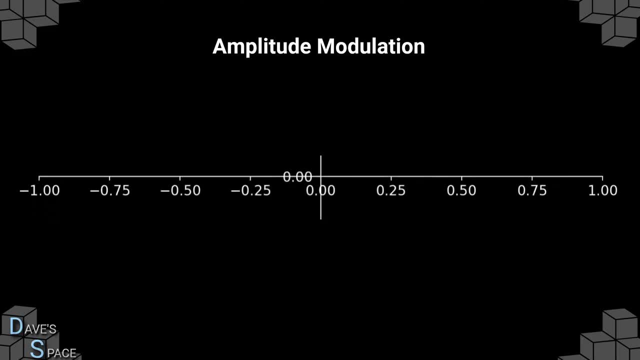 modulation signal. so for a simple binary zero and one you could imagine we have, the possible amplitude of the modulation waveform can be either zero, or one representing zero or one. and so for the modulation frequency, which is how often we switch our bits of zero and one, we are sending one bit per symbol. symbol here means: 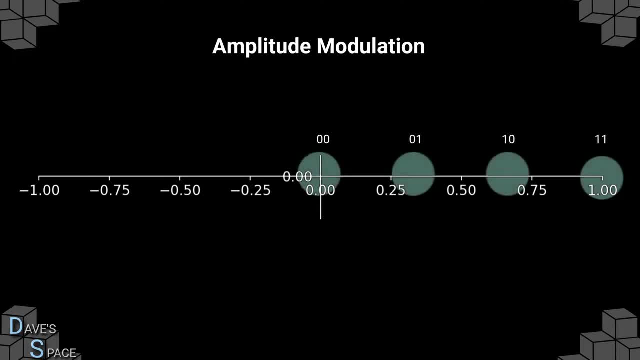 per modulation time period. instead, you could define multiple amplitude levels. so, for example, you could not just choose zero and one corresponding to min and max our amplitude. you could choose intermediate values, in which case, when the receiver sees these intermediate values of amplitude, you could assign them different symbols. 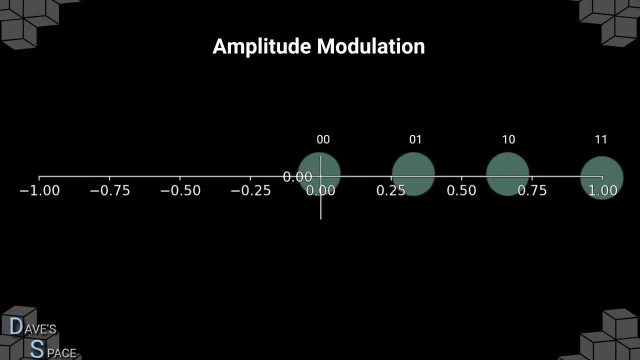 so, for example, in this case we would have four distinct states, so you can call this two bits per symbol. so for every change in modulation we convey two unique bits. now for quantum, this is very similar, but rather than being a one-dimensional amplitude modulation, two-dimensional amplitude modulation. 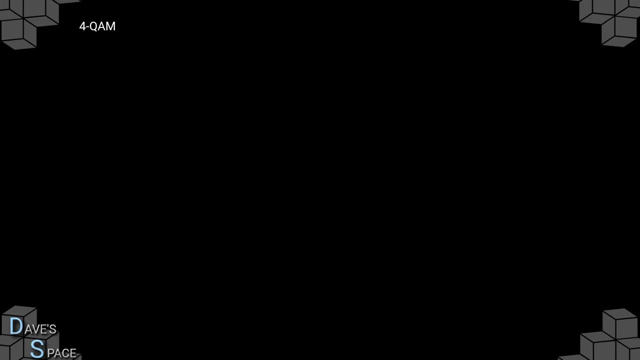 So, for example, if we look at a four QAM, which is a way of expressing the total number of states available, we have a constellation diagram like this. We can see that for the I of T carrier, which remember was the carrier in our case. 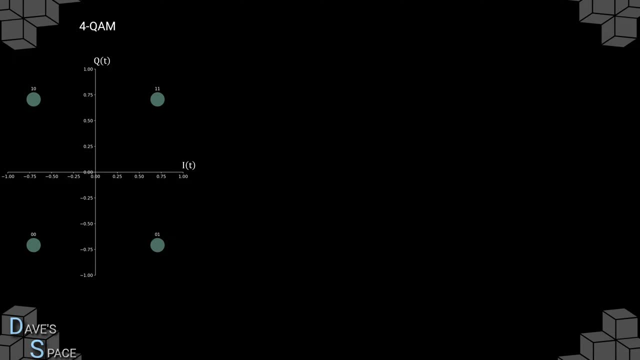 that was multiplied by cosine, we can see that we have two possible amplitudes. Here. the amplitudes are around minus 0.75 and 0.75.. Likewise the Q amplitude signal, which was the one multiplied by sine. 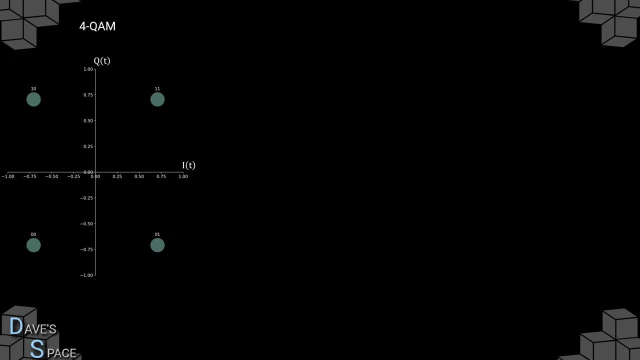 also has two amplitude states, which are also approximately 0.75 and 0.75.. Now the advantages of QAM is that we can pack more of these states into our constellation diagram. So rather than just having two bits per symbol, we could move to some high level QAM, such as 16 QAM. 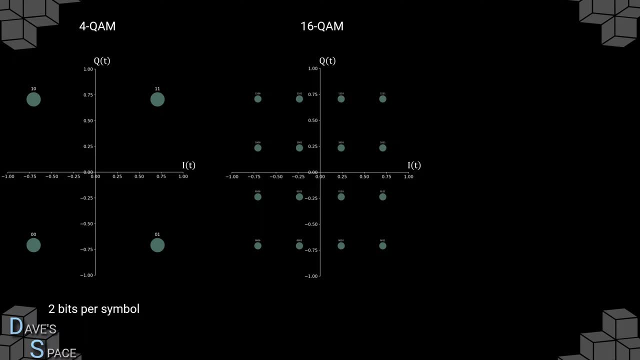 In this case it's possible to fit four bits per symbol. So you can see here we have a total 16 states available. So for the I of T channel, we can see we have four states around minus 0.75,. 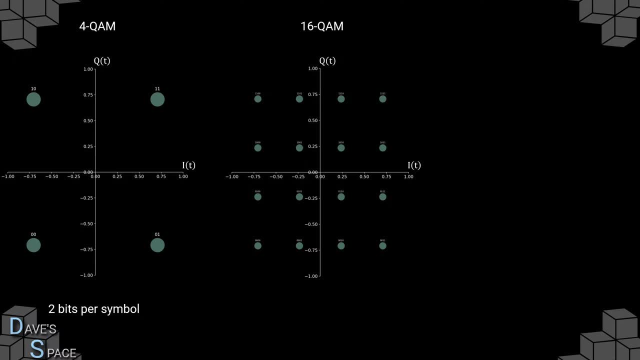 minus 0.25,, 0.25, and 0.75.. Likewise for the QT channel, we also have those available states. So by choosing unique combinations of the amplitude of I of T and Q of T, we can select different symbols. 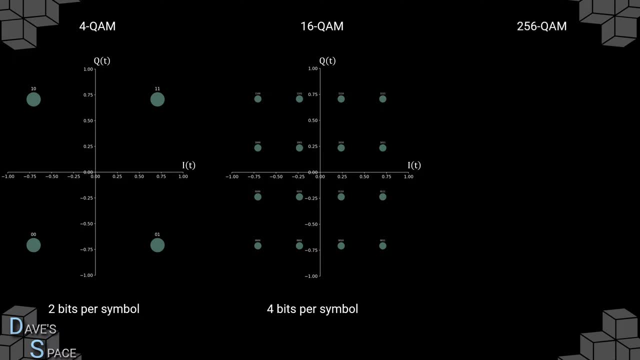 which will give us four bits per symbol. Lastly, we can fit even more of these onto our constellation diagram by going to higher levels of QAM, such as 256, in which case we have a total of 16 amplitude states, both the I and Q of T channels. 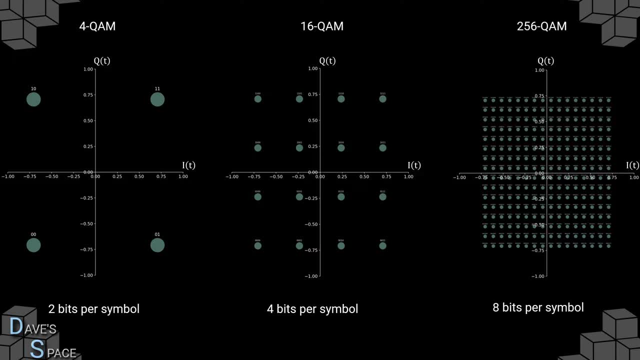 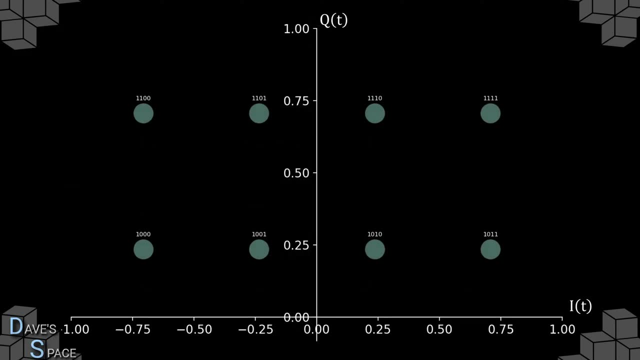 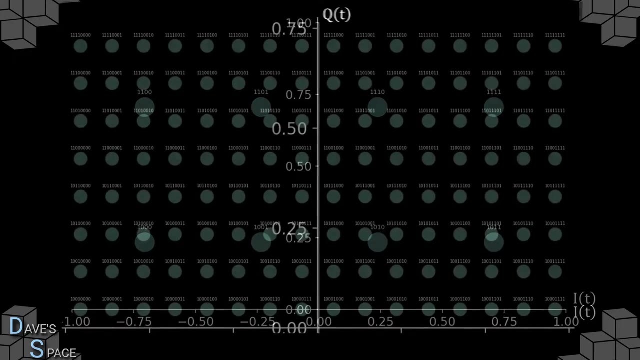 With this particular system, we would be sending eight bits per symbol, And so, taking a closer look, you can clearly see here all the different amplitudes of I and T and Q of T correspond to different bit values, And likewise for the 256 QAM. 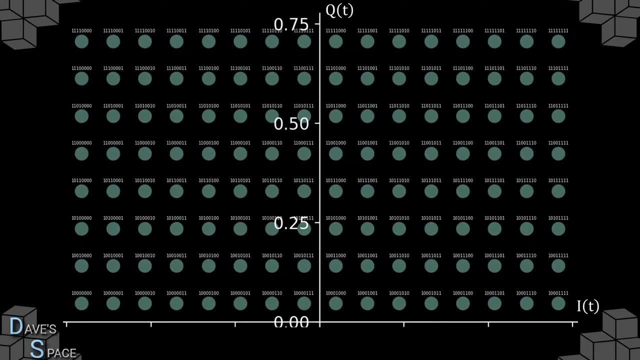 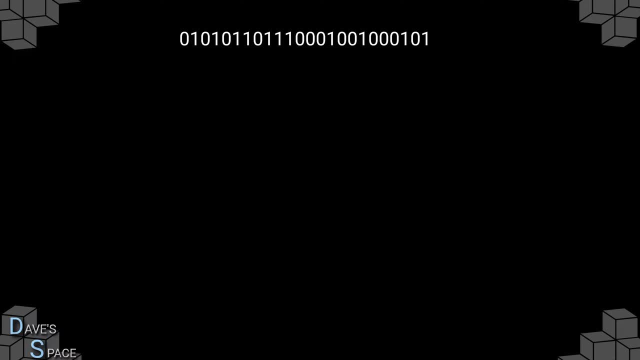 we can see eight bits per symbol. Now let's have a look how we would send this information. So imagine you have a bit string like this that represents some data you wish to send, And then for four different types of modulation. so simple: amplitude modulation. 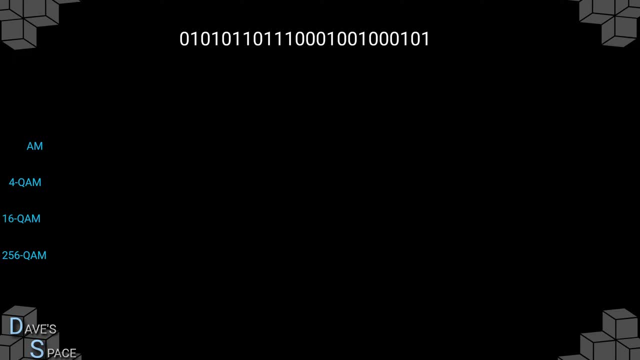 a 4 QAM, 16 QAM and 256 QAM, And this is just a bit, And so that's what we're going to be doing. At some period of time, we'll be switching our state depending on the data to send. 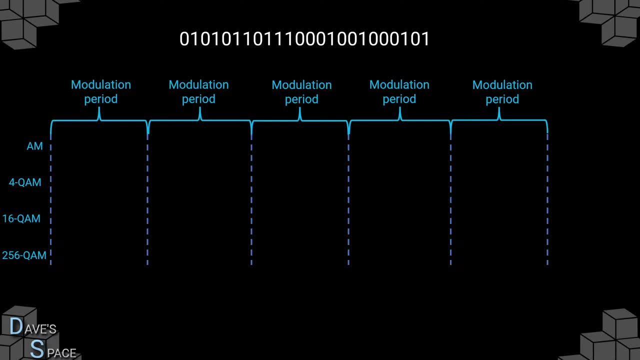 which will be known as our modulation period. And so for simple amplitude modulation, we simply have to look whether the bit is 0 or 1, and then change the amplitude accordingly. For a 4 QAM, what we have is four possible states. 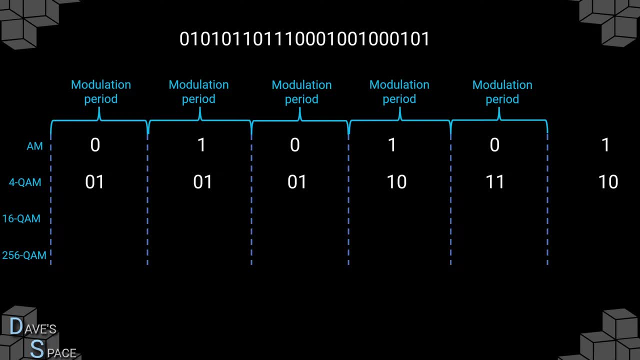 because we have two bits per symbol. Depending on the state, change the values of i of t and q of t. Likewise, for 16 QAM we have more symbols which we can send and so the amplitude states of both i and t, of q of t will be different and the 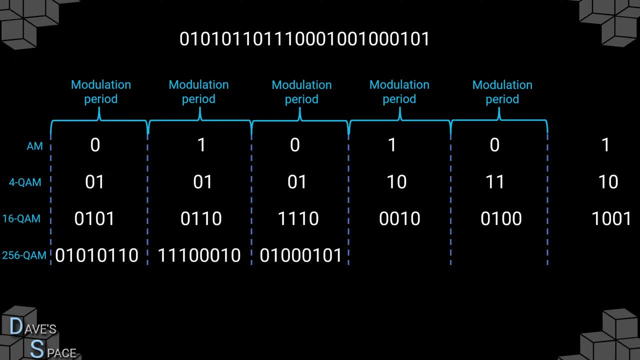 same for 256 QAM, but this time we have 8 bits per symbol, And you'll notice that within the same period of time we can send more information with the higher levels of QAM. So this entire bit string here can send in just three of our modulation periods using a 256 QAM. what 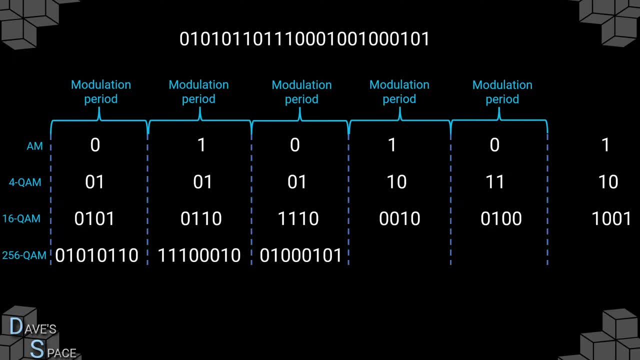 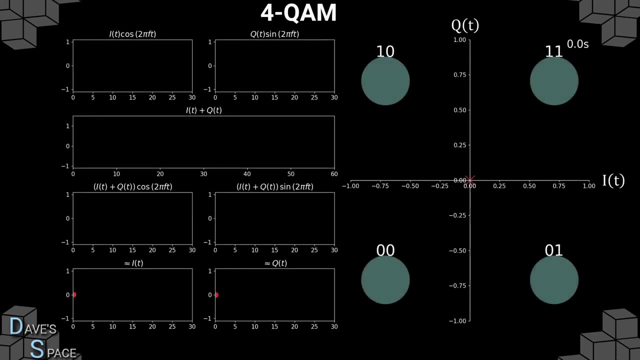 requires 6 modulation periods using a 16 QAM, 12 using a 4 QAM and 24 using amplitude modulation. So lets look at a more interesting example. So what I have here is an animation showing a 4 QAM system. On the top left we have the two independent carrier waves which have a 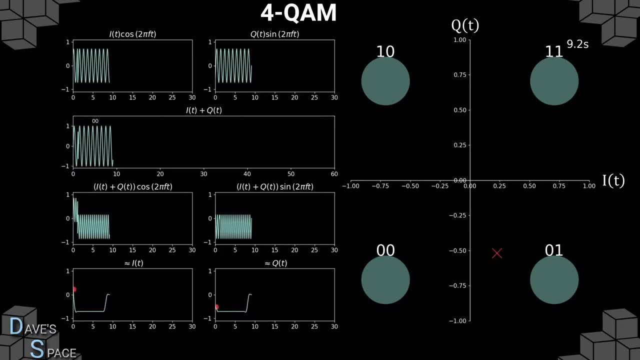 been modulated. So these are our modulated carrier waves, our I of t and our Q of t signals, which have been multiplied by cosine and sine respectively. The next graph on the left is the summation of these two. You can see it just looks like quite a random assortment of sine and cosine. 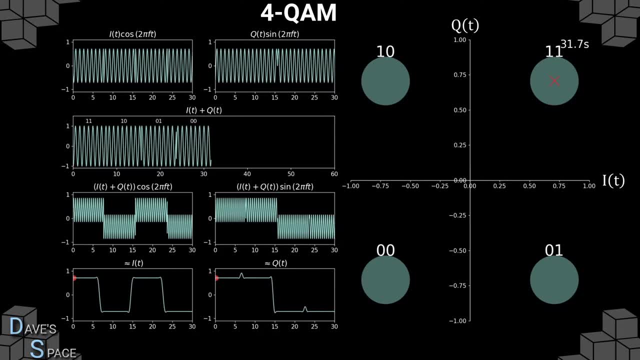 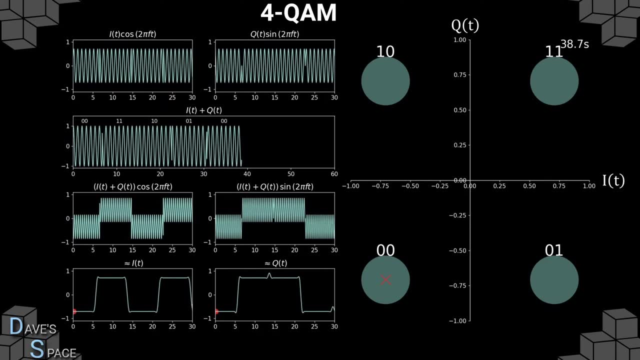 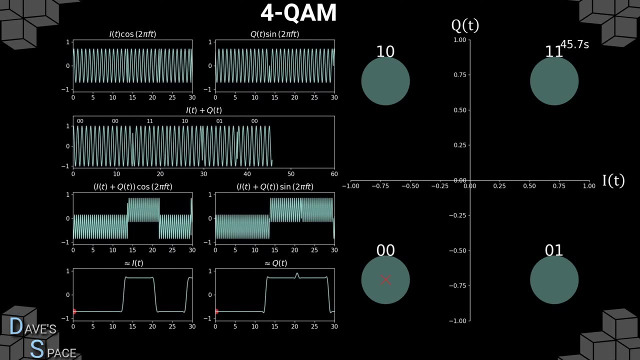 The two plots below. that are the interesting parts. so here is where we perform the coherent demodulation: On the left we multiply by cosine, on the right we multiply by sine and then, after just a simple filter operation, to filter out the frequencies at twice the carrier frequency. 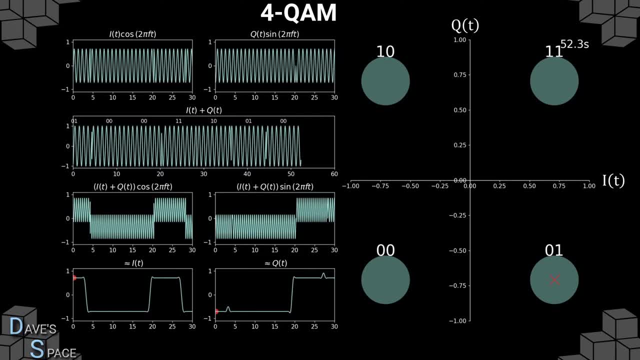 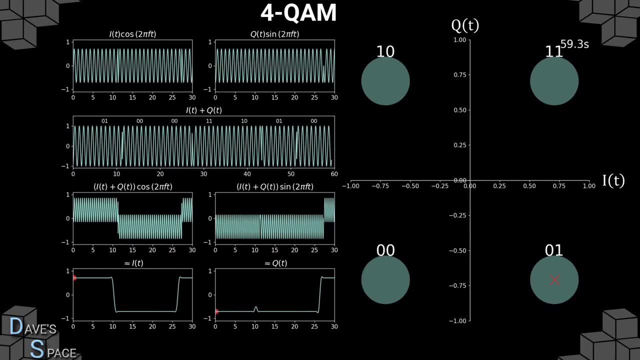 we can see that we end up recovering a signal at the bottom. These signals are the I and Q modulation amplitudes which you can see on the right we are tracking. So you see, here we're currently looking at the bit 011.. 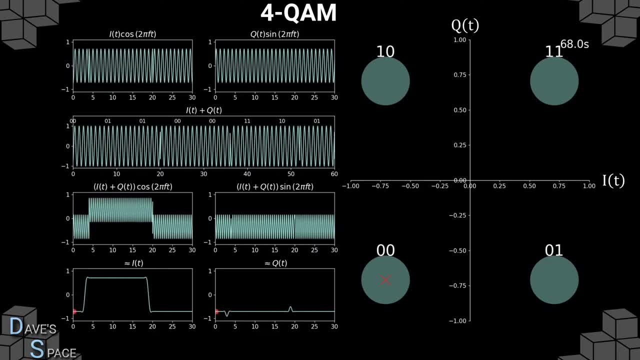 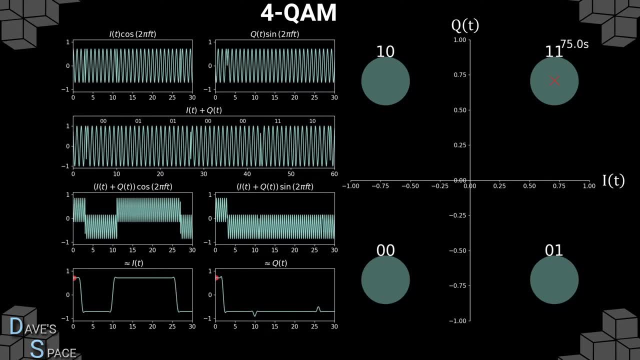 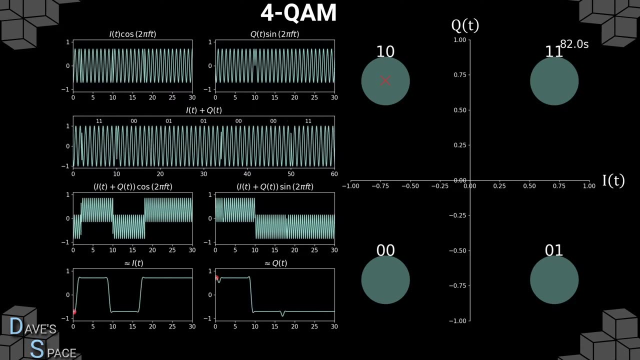 Which has now switched to 00.. 00 is achieved with an IT amplitude of minus 0.75 and a QT amplitude of minus 0.75, which you can just see. We now switch over to another bit, which you can see, now 10.. 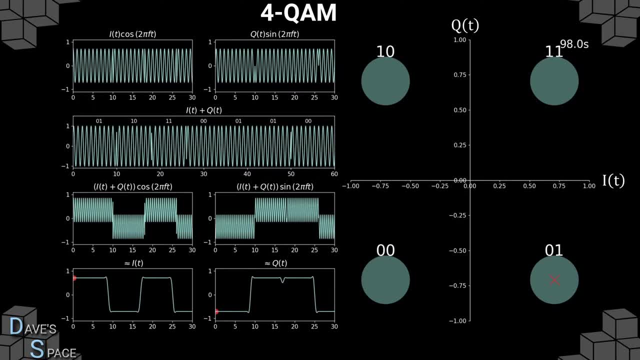 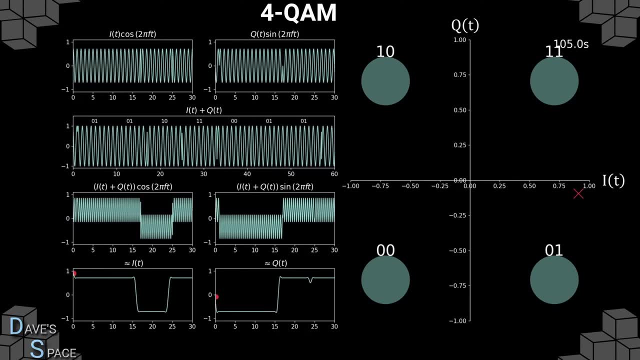 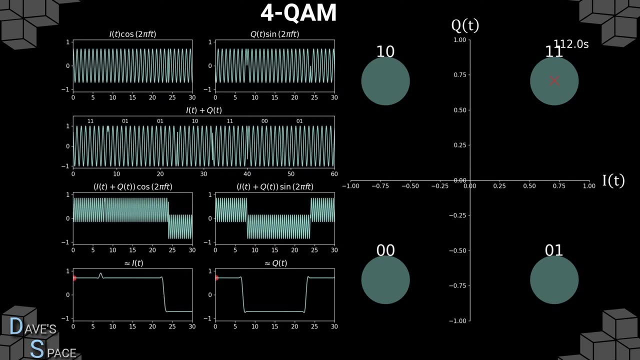 And you can see we can keep going like this. So for every unique bit symbol, we see that we're basically extracting the amplitudes of the I channel and the Q channel independently. So for the bit 01, I must be 0.75 and Q must be 0.75, which you see here. 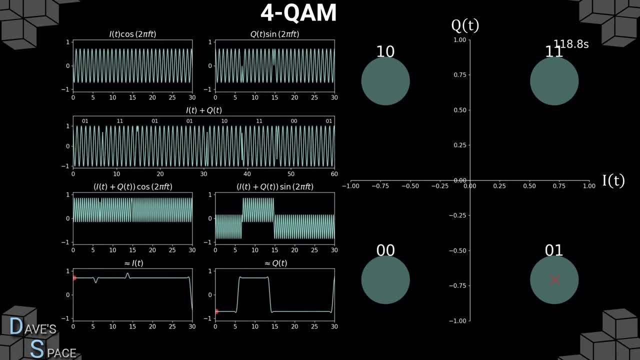 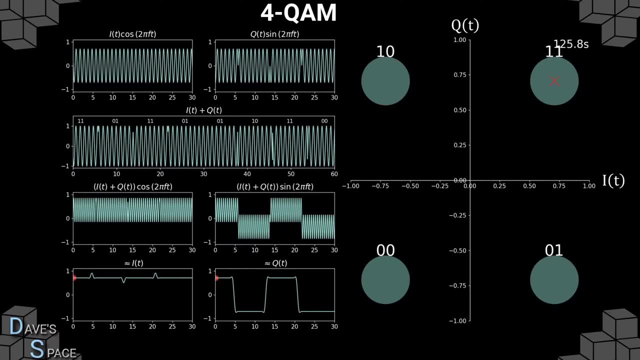 Now I has remained at 0.75, but Q has changed to minus 0.75,, which we can clearly see on the left: 00. 00. And our state, which is around every seven seconds. We can see that the bits that we send have changed. 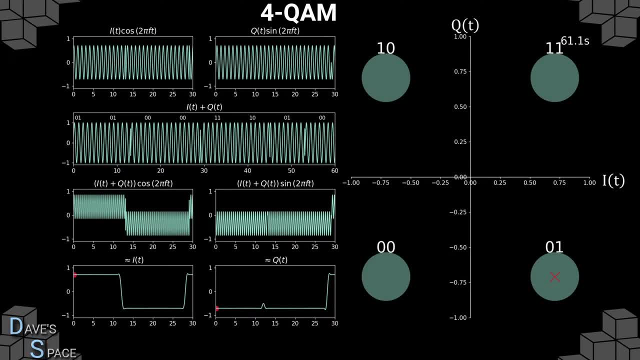 And so this is just a still from the previous animation, So you can clearly see here: our bit of 01 is an I amplitude of 0.75 and a Q amplitude of minus 0.75, which is clearly represented on the filtered signals on the bottom left. 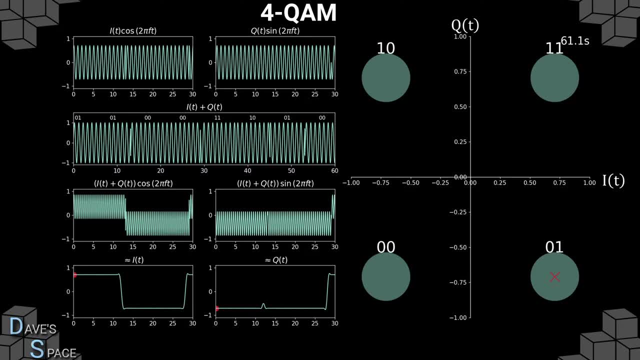 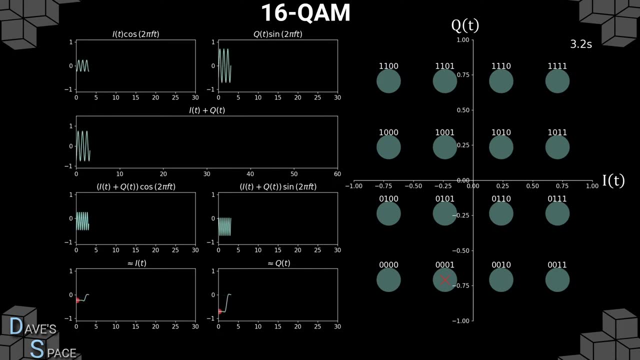 00.. extracted, the information which you can see in the second graph was indeed 0- 1. let's have a look at some higher level QAM. so for a 16 QAM, we have the following: so instead of sending just two bits per symbol, we're now sending four. 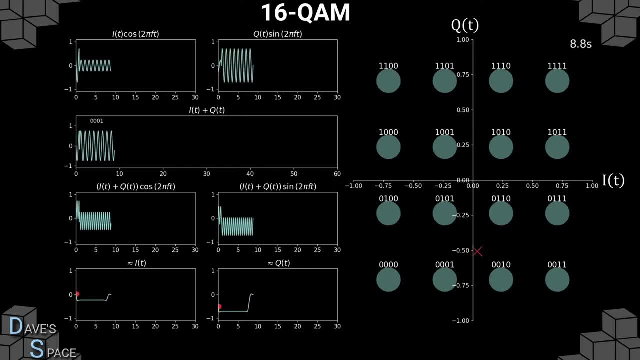 at a time. this gives us more unique amplitude states which we can send. so you can see on the receiver on the bottom left we're now receiving up to four possible levels of amplitude for both the I channel and the Q channel. these four levels can then correspond together to one of the bits on the 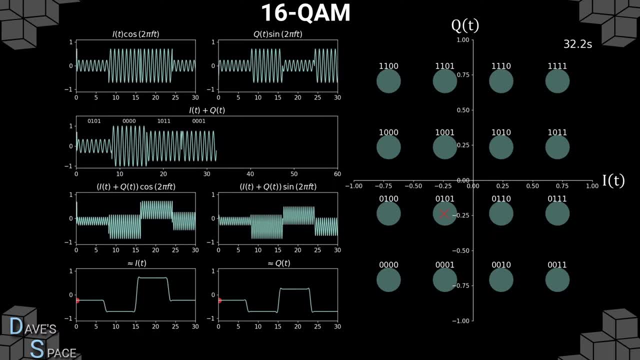 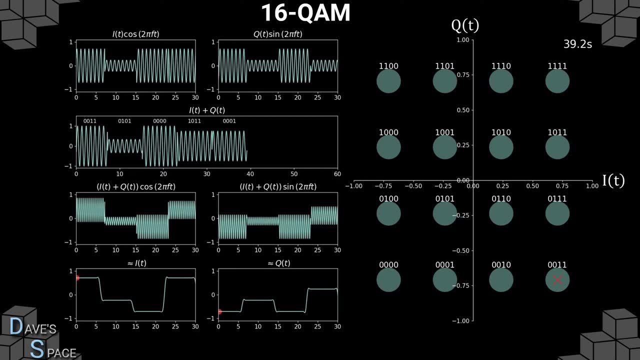 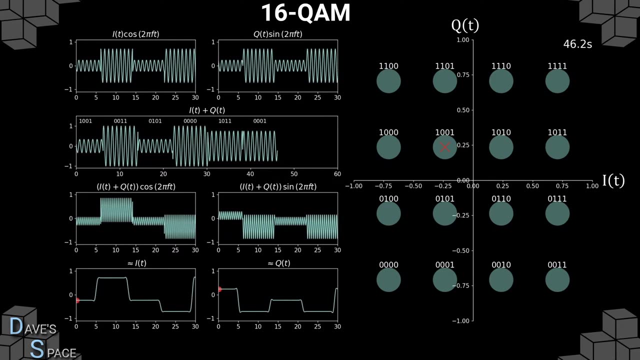 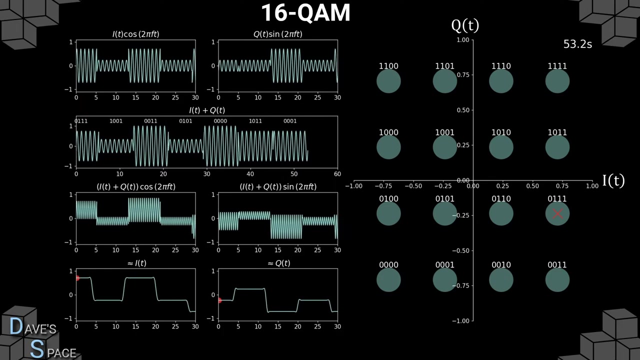 constellation diagram. we're modulating at the same seven second period which we were before. now we're sending four bits at a time instead of two, and so this data will be sent twice as quick as before, and so before, where it took around a hundred and thirty seconds, this should be done in around 65 seconds. 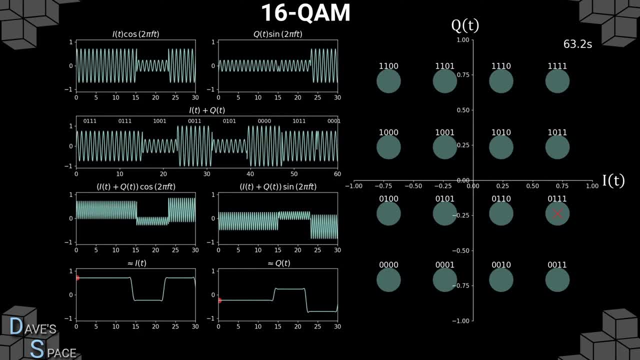 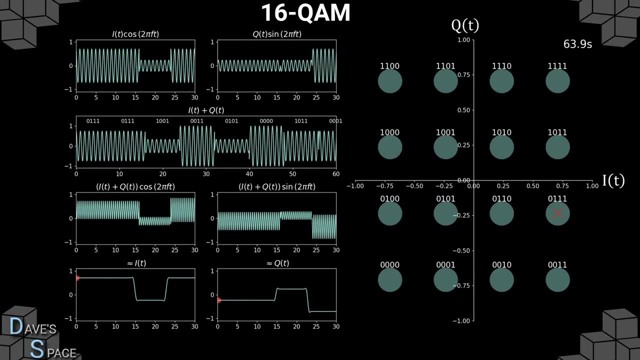 so we should be coming up to one of our last bits now and we can see we're done. so the last bit to send was 0 1 1 1, which is an I amplitude of 0.75 and a Q amplitude of minus 1.75. 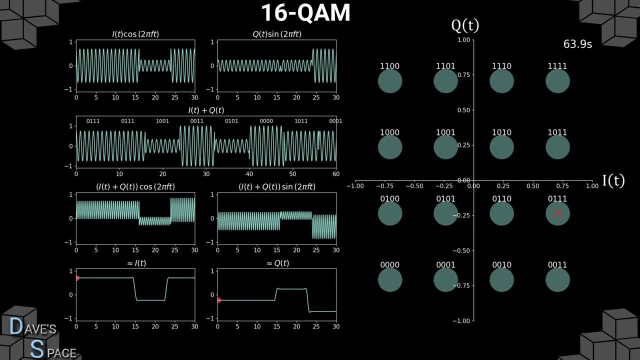 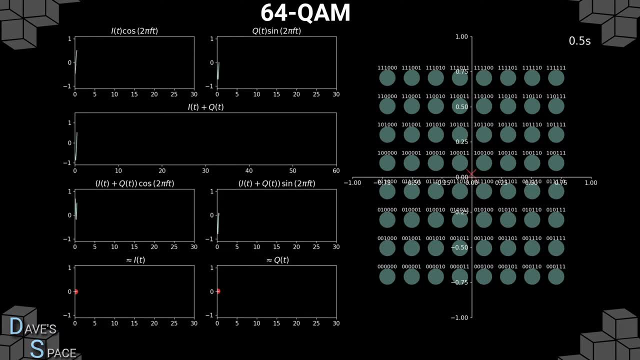 0.25, which we can clearly see on the bottom left. now let's take a look at an even higher level of QAM: 64 QAM. so here we're sending six bits at a time, so you can see, the first bit comes in. that corresponds to an I and a Q amplitude. 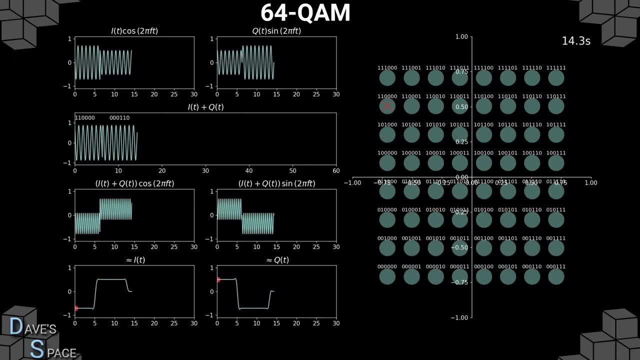 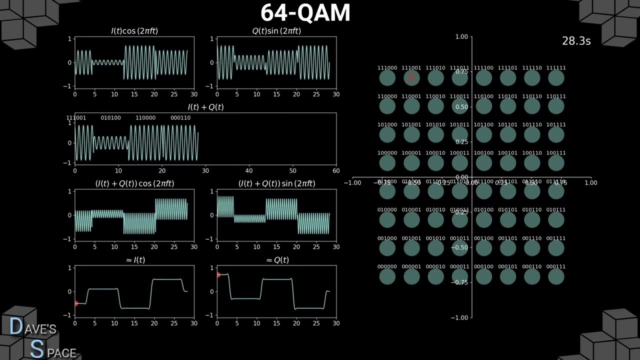 which we can see, that we on the bottom left, where we filtered out our coherently demodulated signal, we can indeed recover those out of the signal, those amplitudes, and extract those bits. and now, because we're sending six bits per symbol instead of four bits per symbol, we should finish sending all of 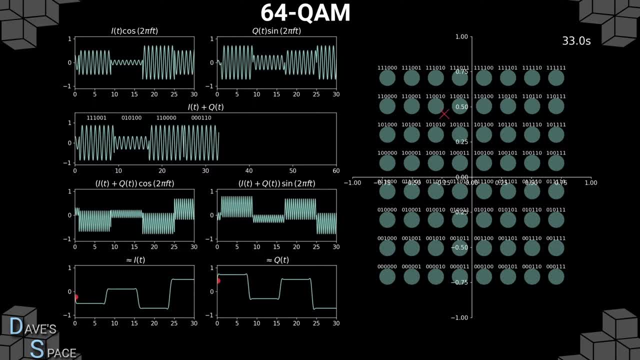 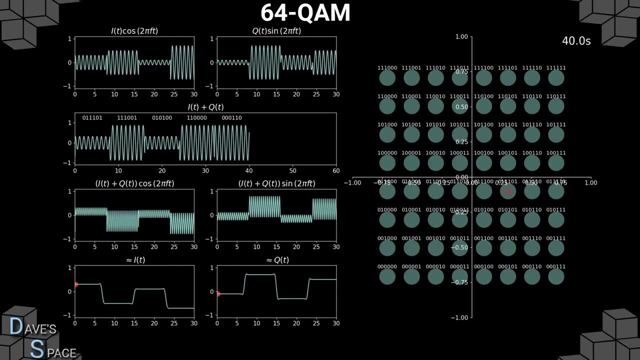 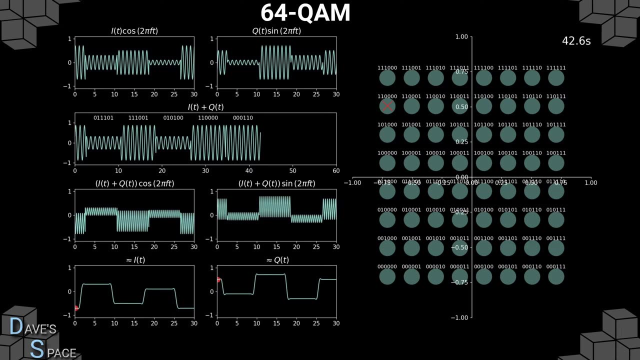 our data quicker than we did when we were sending four bits per symbol. so previously it took around 63 seconds to send all our data. when sending four bits per symbol with the 64 QAM, we send all our data in just 42 seconds. so it's the. 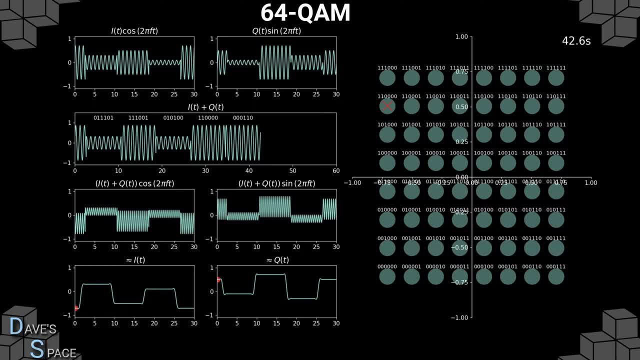 same modulation frequency, the same modulation period, but we're sending more information per modulation using many more levels of amplitude on the I and Q channel. and it's important to know here if we had a lot of noise in our signal: the little red X that follows around the filtered 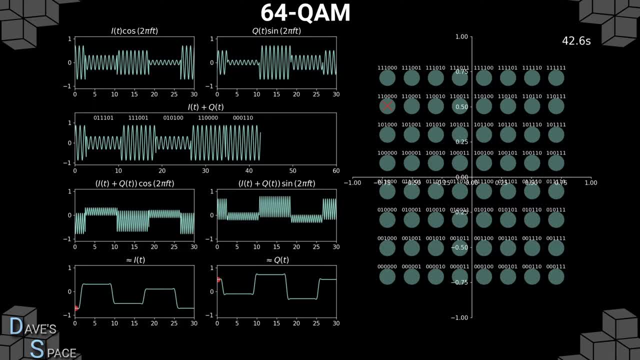 amplitude states would not be so well defined. they would tend to jiggle about on their spot and depend on how much they jiggle on the spot will determine how close we can put our values in the constellation diagram. If the values are too close then we could misinterpret some simply because of 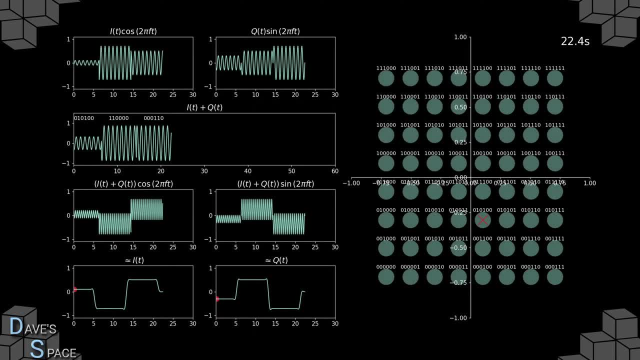 random noise, and so just a still from the previous 64 QAM, we can see that our original signal was 010100, which is an I amplitude of around 0.1 and a Q amplitude of around minus 0.3, which you can see is: 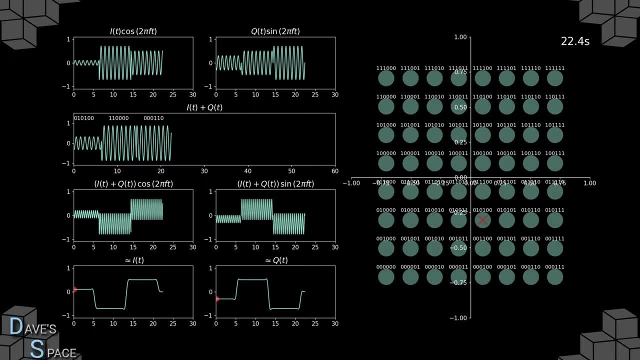 being picked up by the filter signals on the bottom left. So we can really see now, by choosing more bits to send per symbol, which results in more amplitude levels above the I and Q channel, we can send more bits during the same modulation period, meaning we can send more bits in the same 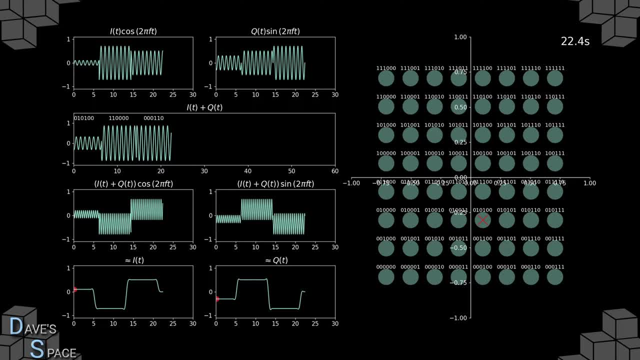 period of time. so, where a simple amplitude modulation would require us to send our zeros and ones faster, which would require us to have a higher frequency carrier wave in order to handle the high frequency modulation wave, WAM does something different by changing the number of amplitude levels of two quadrature signals in order to send more data. so 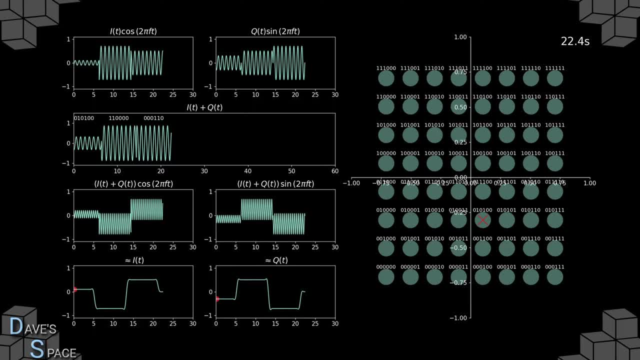 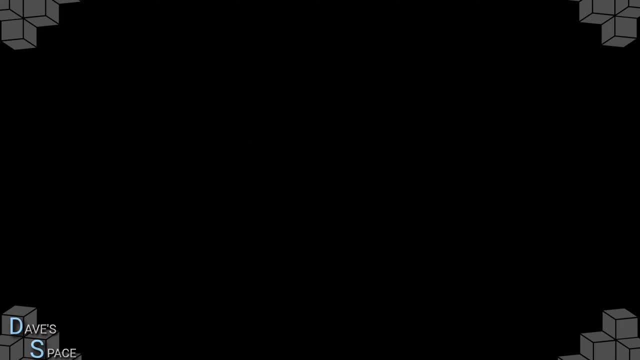 has clear advantages in terms of the ability to send data on lower frequency carrier waves. So let's just talk about filtering. Let's say we have a quadrature amplitude modulated signal consisting of two independent waves. so here we have our I channel and our Q channel and here we're modulating at 7. 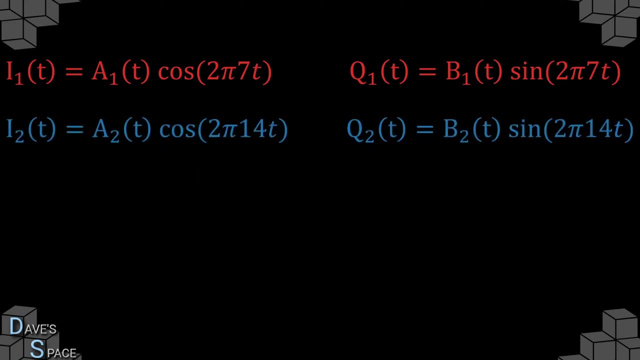 Hertz. Let's say we have another independently modulated QAM signal. so here an I2 and a Q2 signal, independently modulated by an A2 and a B2, but this time at 14 Hertz, and finally we have a third independently modulated quadrature. 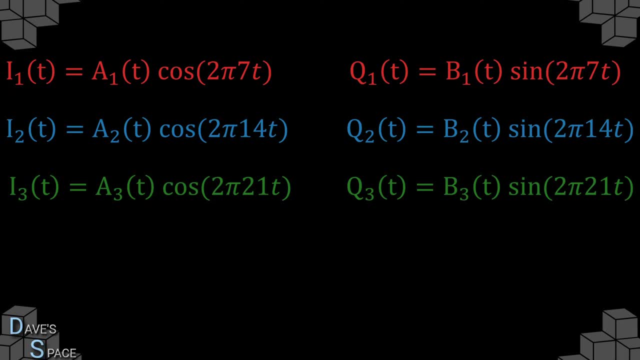 amplitude modulated signal I3 which has a carrier frequency of 21 Hertz. So the Fourier transform for these three signals is given as follows. So you can see here that the modulation signals A and B is information in the frequency space located around the carrier frequencies of 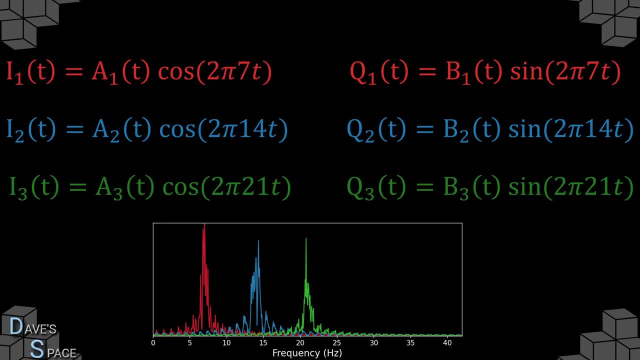 7,, 14 and 21 and we can see there is some overlap between the two. so where are the information for the A and B signals? on the 7 Hertz? in red, You can see how that overlaps with some of the A and B signal on the 14 Hertz in blue and. 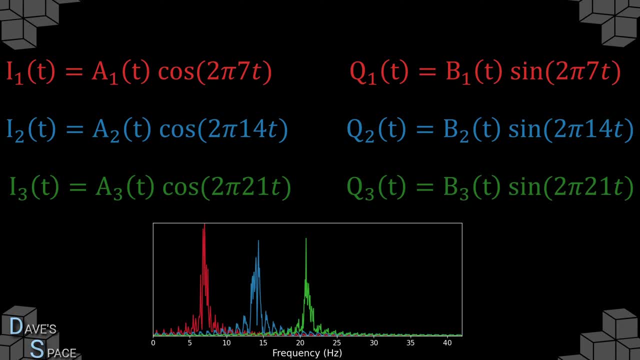 likewise the green, But just like amplitude modulation. if you saw my last video, you would have seen that it was no problem to use different carrier frequencies, modulate these independently, because our demodulation process always successfully extracted the amplitude modulated signal. Well, the same goes for QAM. So let's have a look. if we add all these, 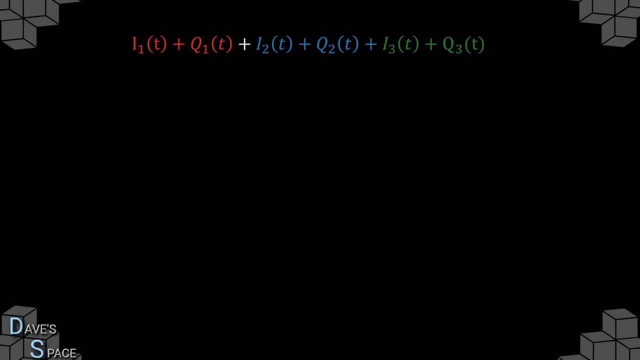 signals together, we end up with our signal out. Now I won't write the math for this because it's a very long equation, but imagine we take our total signal out and multiply it by cosine and sine, both at 7 hertz, cosine and sine, both at 14 hertz and cosine and sine at 21 hertz. We can then use the 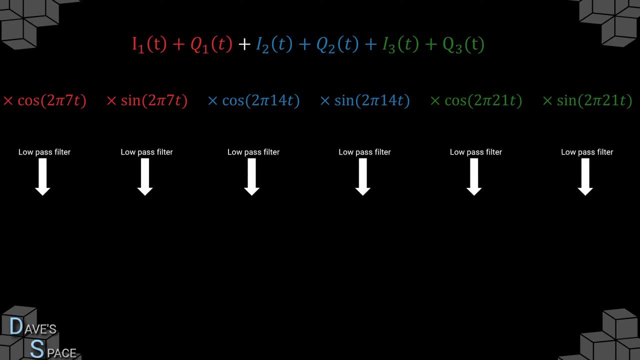 same low-pass filter and all of this data, and yet what we find is that we're able to extract individual modulation signals that were applied to the signals before, Independent of their carrier frequency. So we can still recover both the cosine and sine components A and B for each of the individual frequency components that we sent out. Let's take a further. 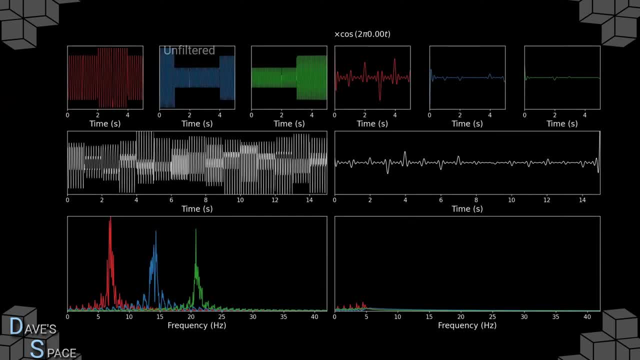 look at this and hopefully make it more clear. So on the left we have our unfiltered signals. on the right we have our filtered signals. What we're going to do is we're going to multiply everything on here by cosine of 2 pi f of t and we'll be changing our frequency. 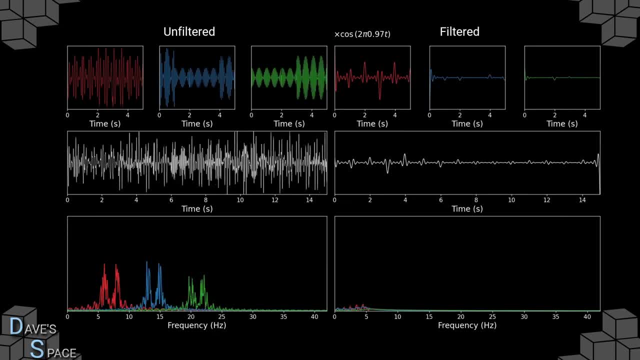 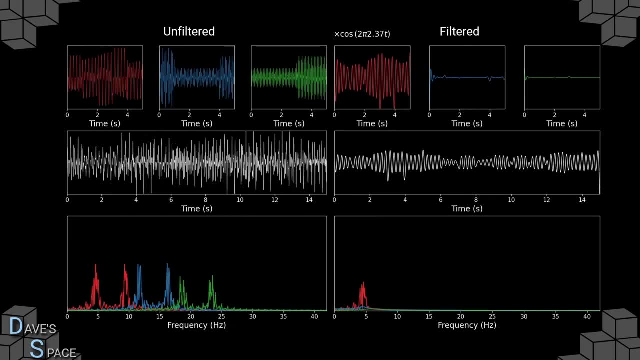 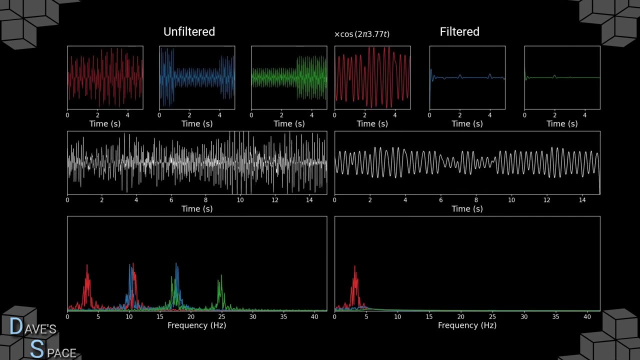 So on the left here you can see that our unfiltered signals multiplied by cosine result in some crazy looking signals. Likewise, the total signal in white also starts to look crazy. But the main thing to watch for is the Fourier transform. on the bottom You see that as we increase the frequency of the 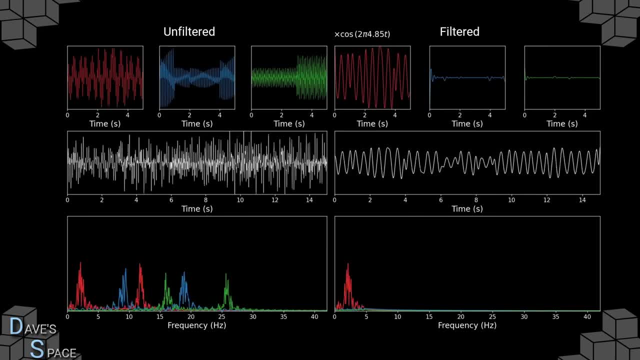 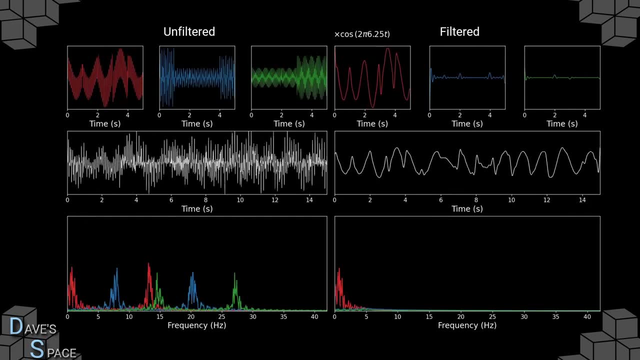 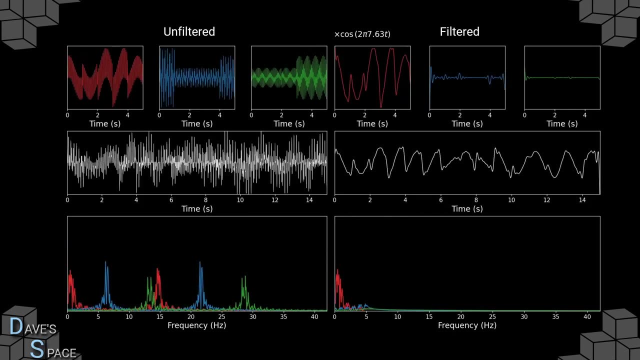 cosine that we multiply our signals with, we start to separate out our frequency components in the Fourier space, And so when we approach 7 hertz, what you'll see is that we're going to have a signal in red is now centered around 0 hertz. This means that we can extract our original 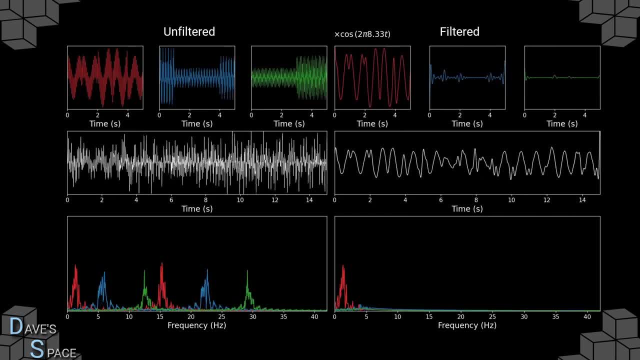 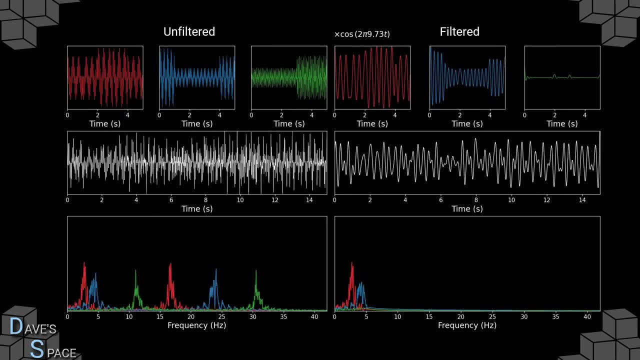 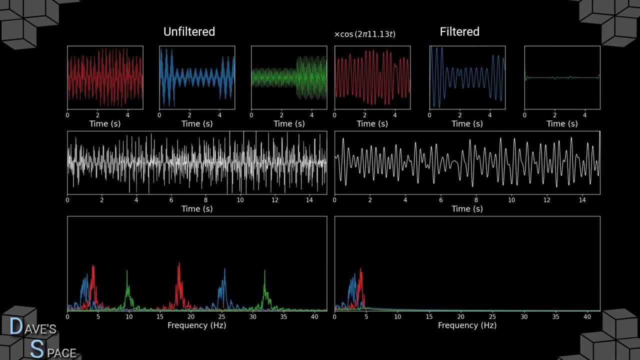 information. so our original modulation wave from this signal by the simple use of filtering. So let's take a look again Now. watch the blue curve on the bottom left, which is our Fourier transform for the 14 hertz signal. As we times this by cosine of 14 hertz, you'll see that the 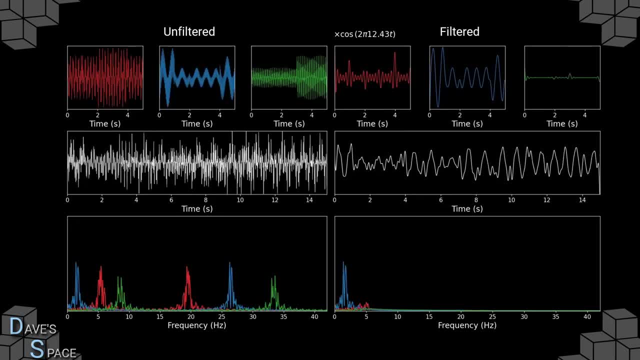 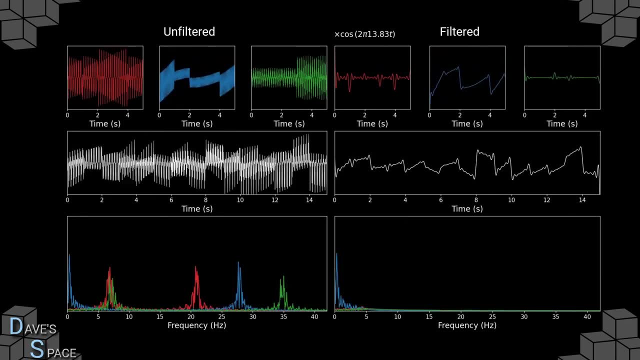 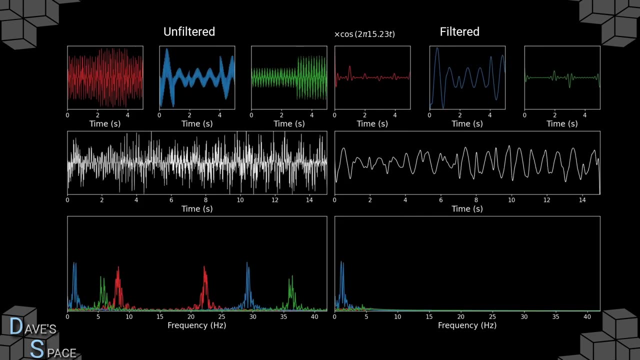 signal- filtered signal on the right in white: when it hits 14 hertz will be a recovered modulation wave there, And then this can continue all the way up to 21 hertz, in which we'll extract the modulation wave which was applied to our green 21 hertz signal. 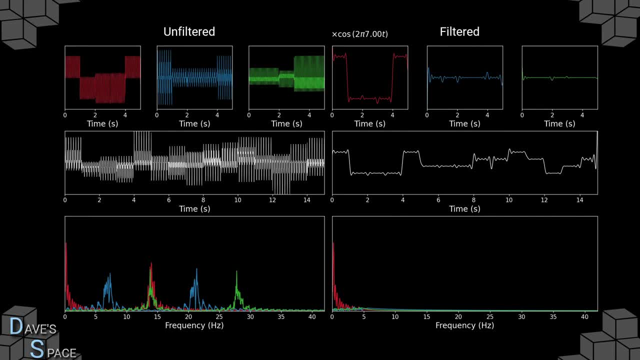 Perhaps if we look here, you'll see more clearly that when we multiply our curves by cosine wave at 7 hertz, Our frequency spectrum on the bottom has shifted everything that is not at 7 hertz to higher frequencies, And the 7 hertz has been shifted towards 0 hertz, And so our 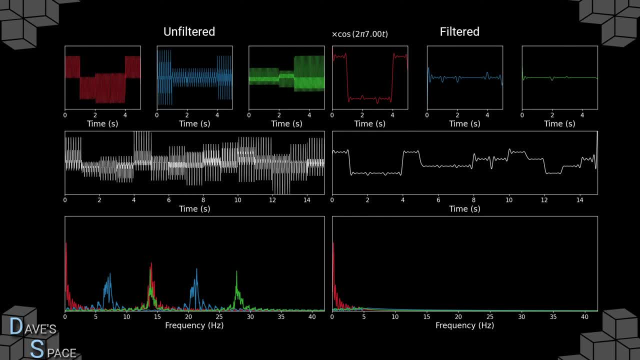 original modulation signal is now centered around 0 hertz, And so a simple filter, which is shown on the right, and then extract a signal which is predominately composed of our original modulated signal that was applied to the 7 hertz carrier signal. in white above is then the original signal that was sent out, which